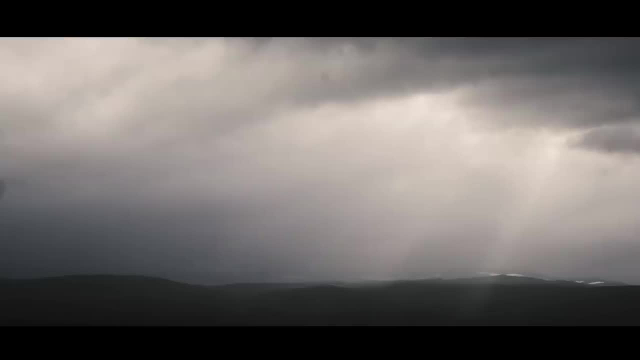 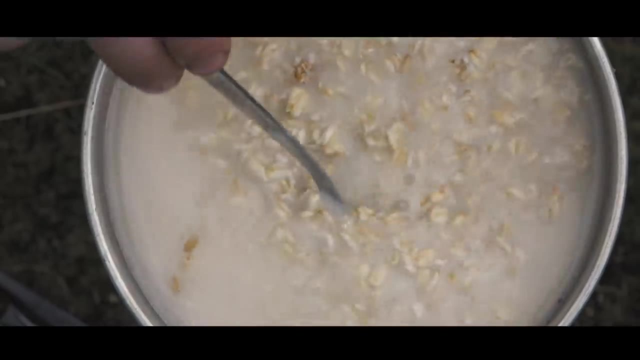 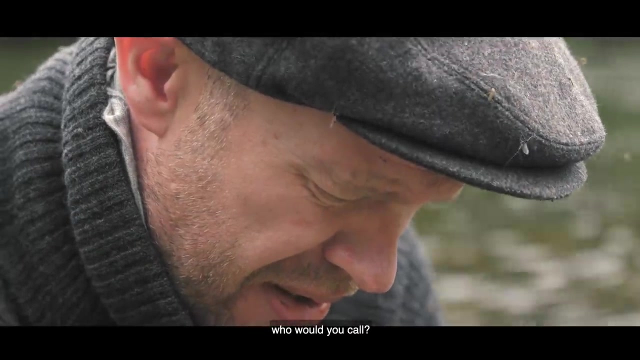 Is a good indication that you are by perhaps the best trout river in Europe. And the trick with porridge is not just to stir all the time. I'm good at porridge. If you were to call a friend and get some tips, Who would you call then? 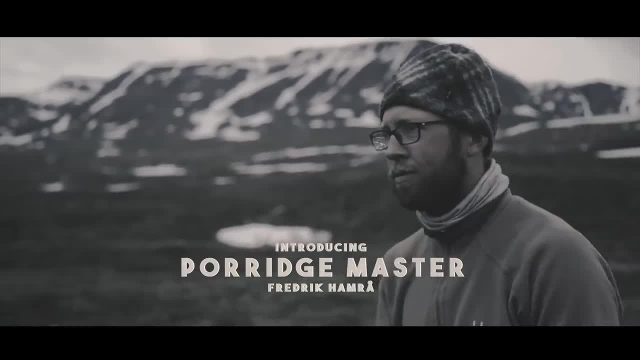 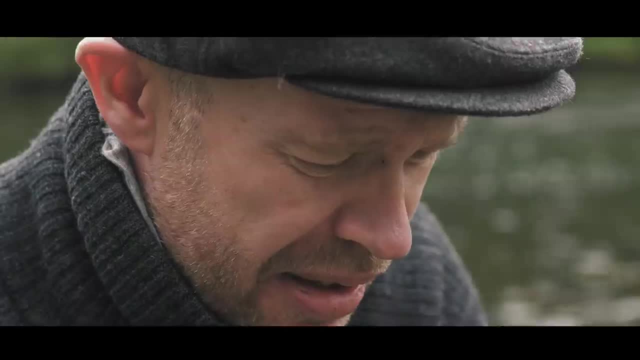 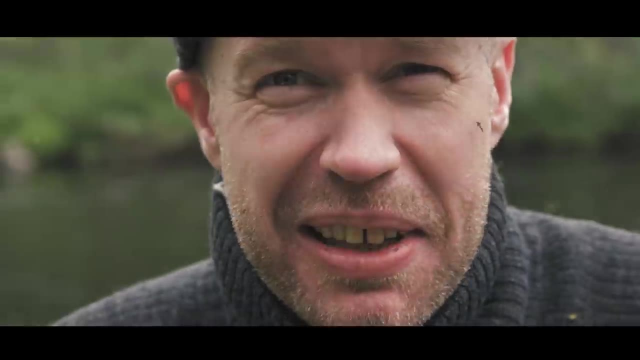 Fredrik Hamloth. I would call Jonsson. He's good, But he also does like Fredrik Hamloth. It's almost a little cheating Because he has some apricots, swiss chard and dates. It's not completely kosher for me. 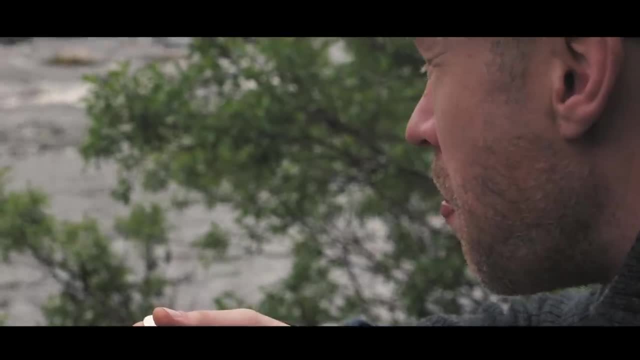 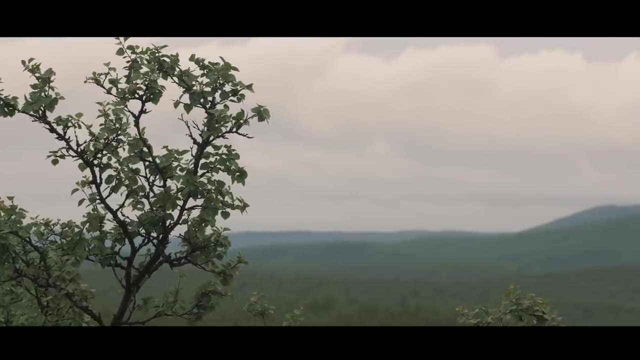 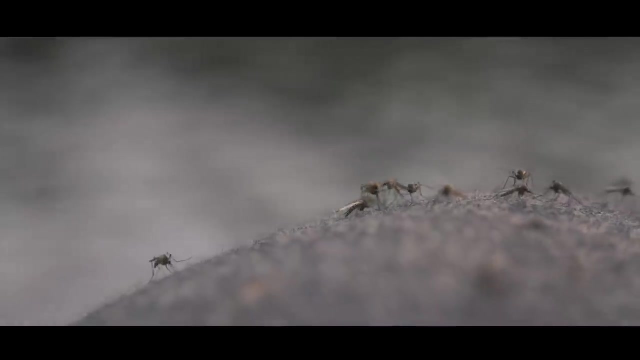 It should be more honest porridge. We were alone by parkey pike, A secret river in northern Finland, And there was no one here to judge us. So after the quite shitty porridge, we decided to have a better dinner. That day a trout would lose its life. 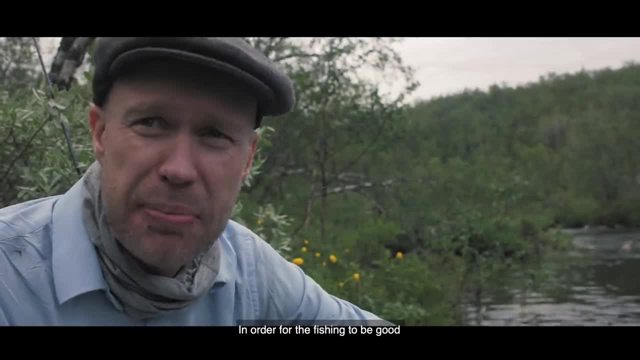 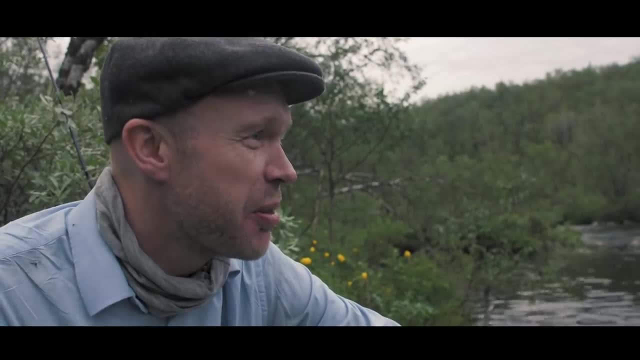 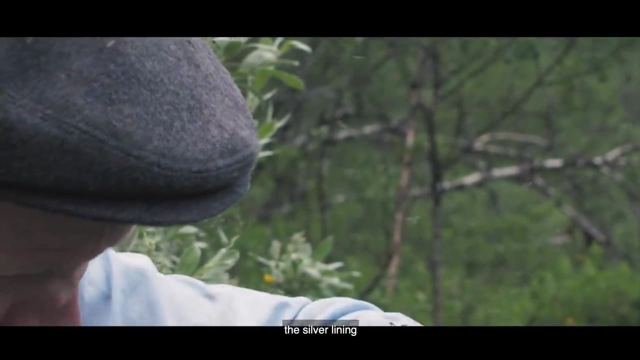 It's a pity that it's like that, But for it to be really good fishing, Really good fishing- It has to be a lot, And we're on our way there now. That's the positive, The silver lining, But it's starting to be quite a lot. 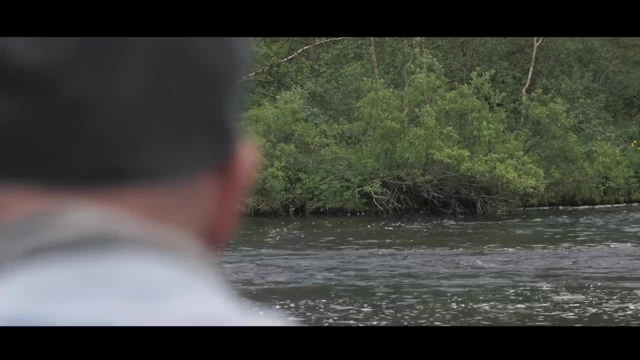 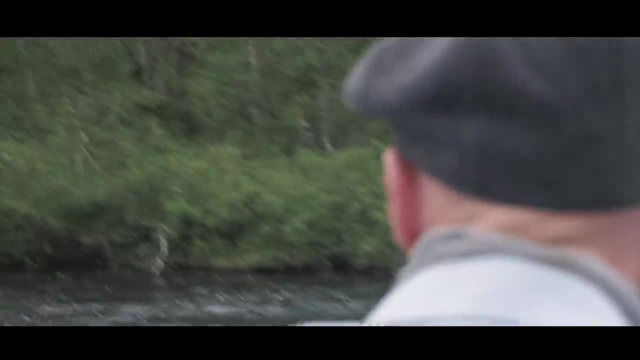 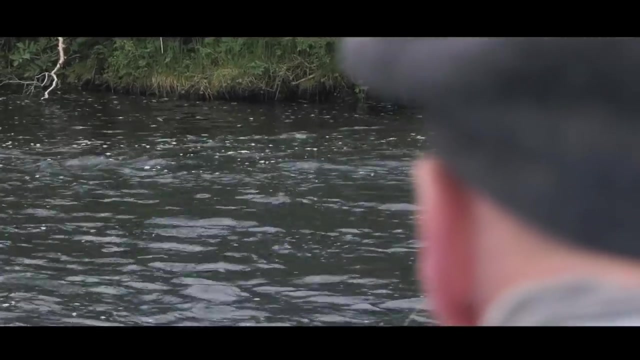 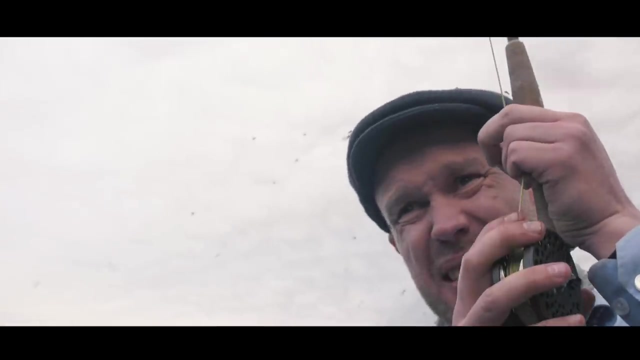 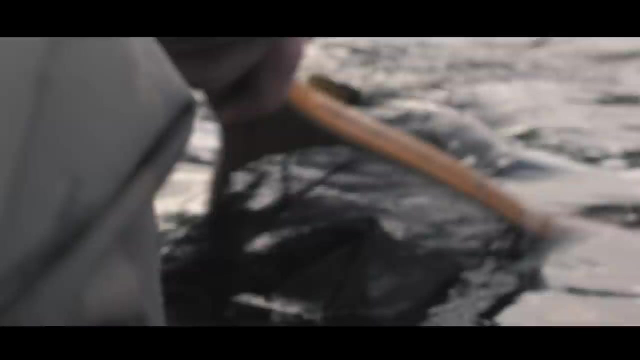 There. Did you see that Up to the right there? Yes, yes, You can see the back. Yes, yes, yes, There it was up in that bush. Oh, it's quite big, It's big. That trout was too big. 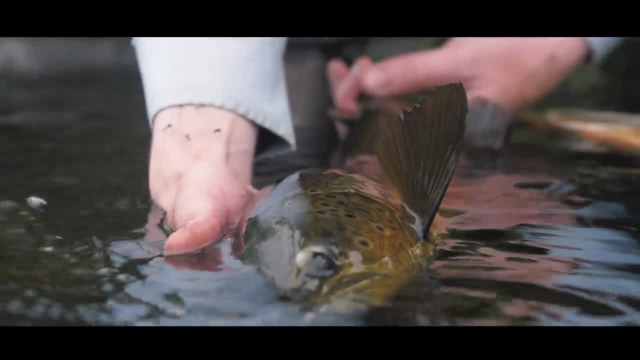 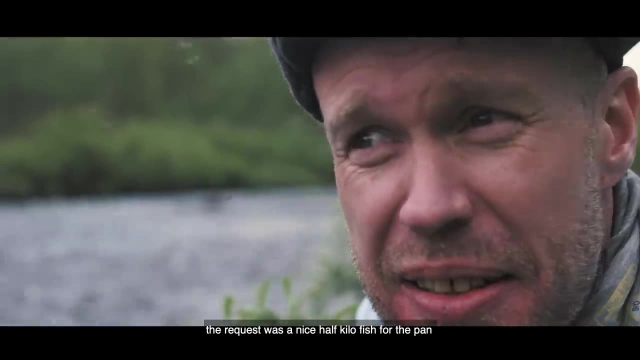 Way too big. We could have fed a soccer team with it, But we were only two men. I know The order was a nice half kilo of char. Then it became two kilos instead. Yes, It's hard to get the small ones out. 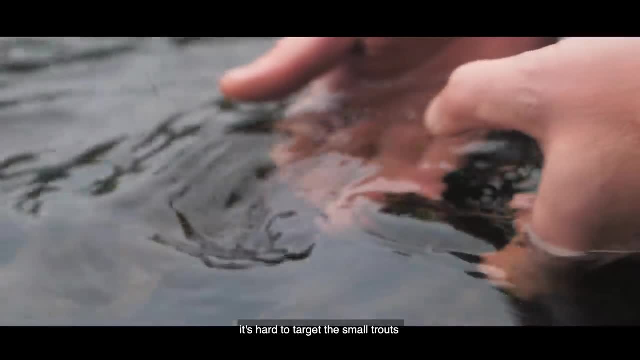 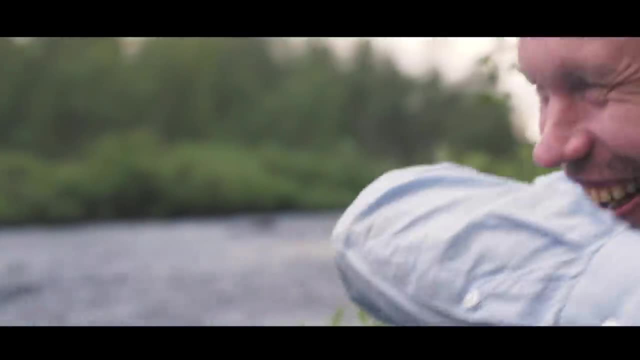 You're a bad hunter. Yes, I'm usually just happy when my friends catch fish, But it had been a while since I caught a trout like that one. It was fun. Yes, It was so good. Yes, it was, It was great. 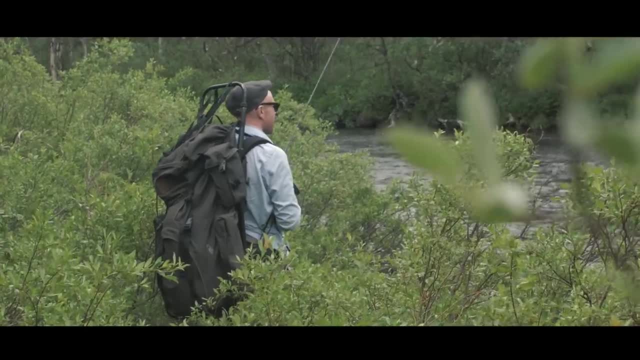 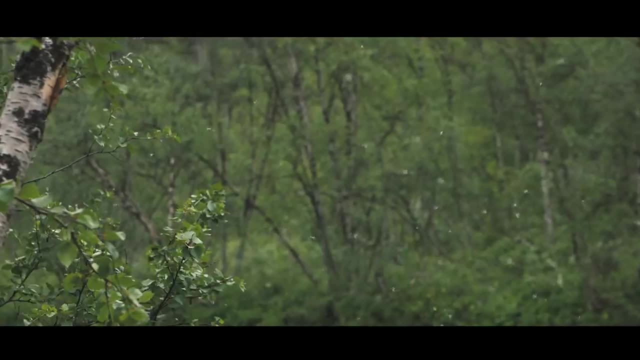 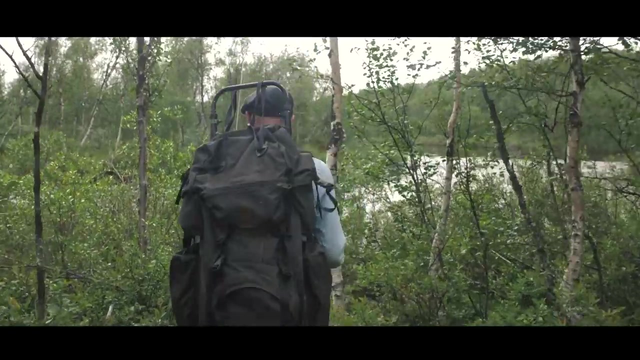 It was a good time. Yes, It was a bit of a bad time. It was a bit of a bad time, Yes, Yes, It was a good time. It was a good time. Yes, Quite a long while, But we were headed upstream. 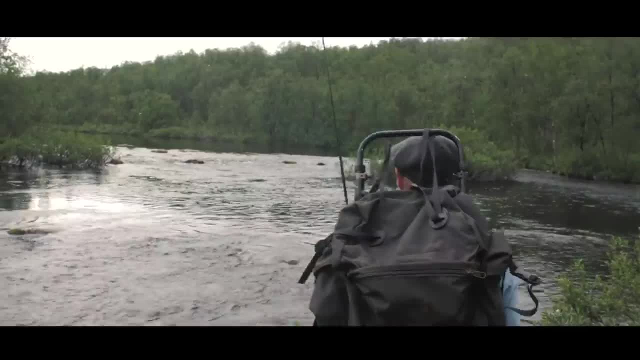 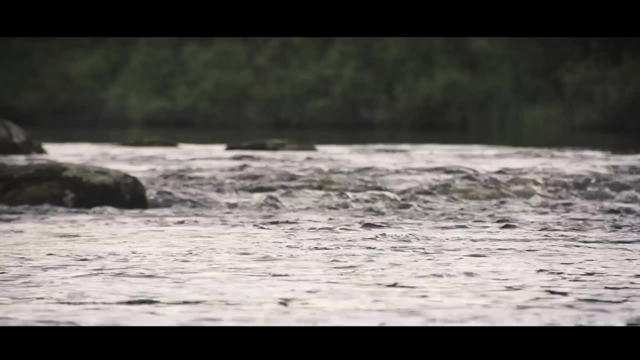 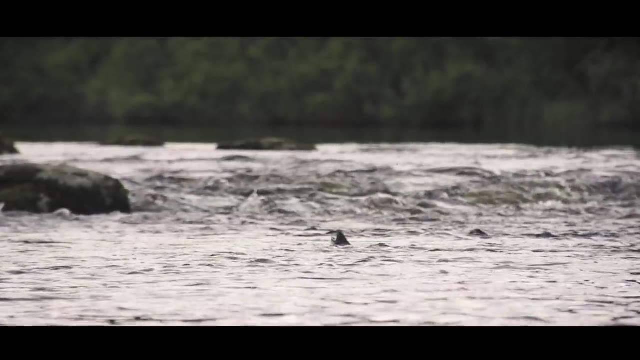 The good thing about sleeping by the river is that you get another chance to fish the pools where you found fish the day before. In retrospect I'm not sure, but in that moment I was sure This was the biggest rising trout I've ever seen. 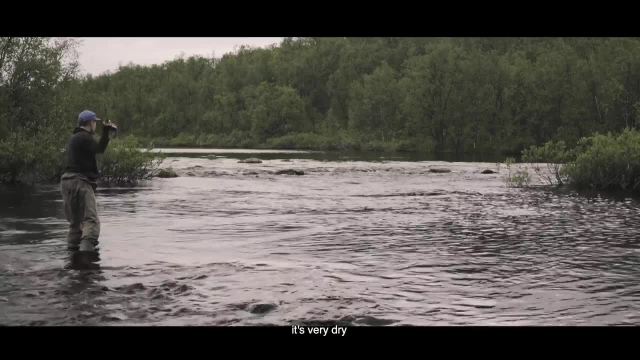 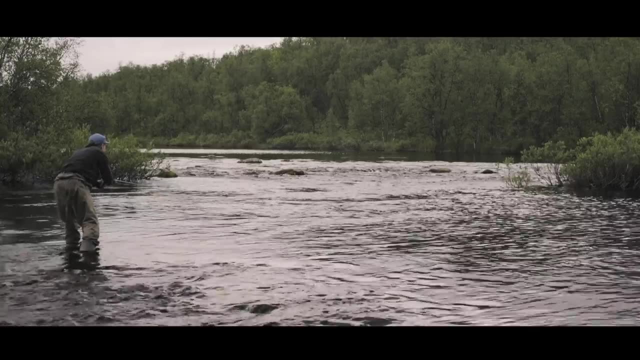 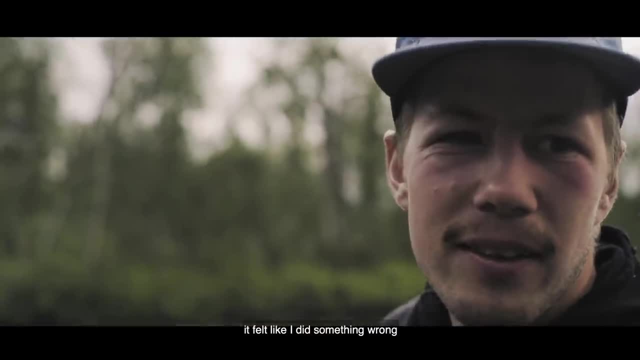 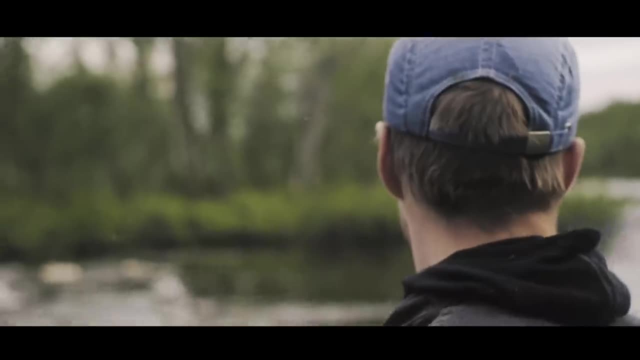 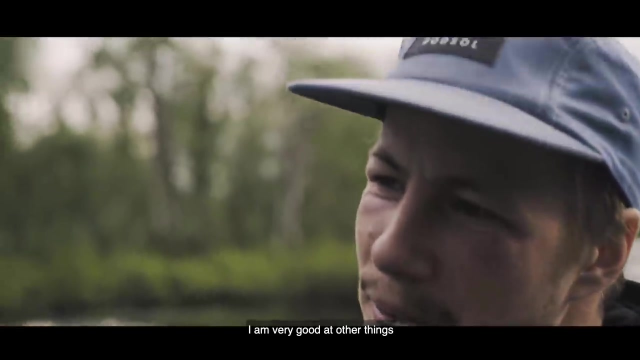 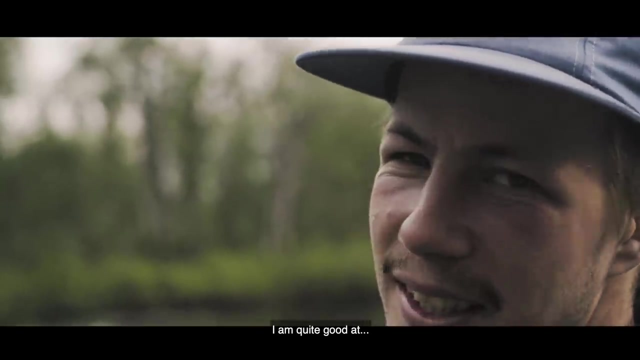 Yeah, that's 1,000 yards. I don't know. It feels like I did something wrong. This is the third biggest fish you've caught here. I don't know. I'm very good at filming waking fish. I'm very good at that And I'm pretty good at taking takes. 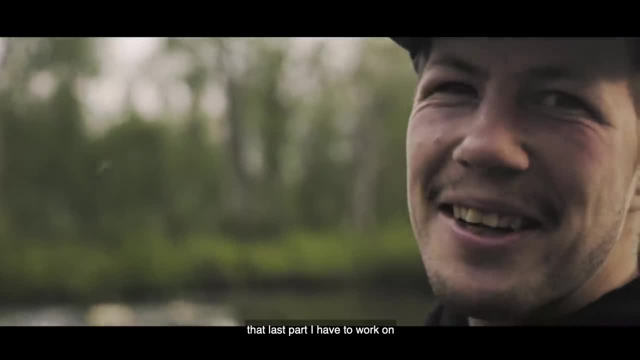 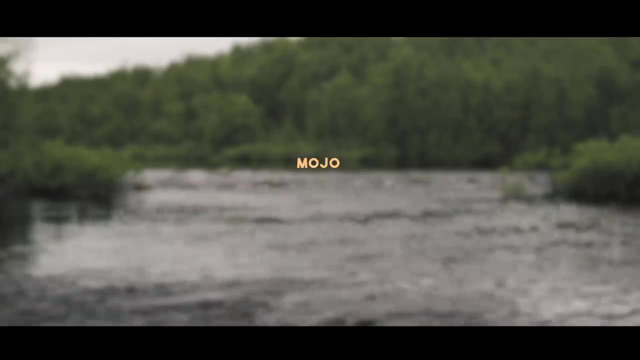 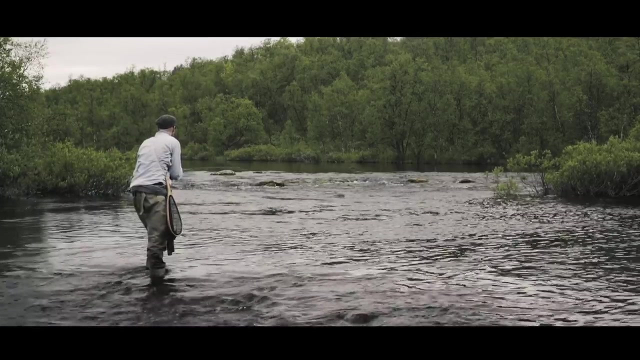 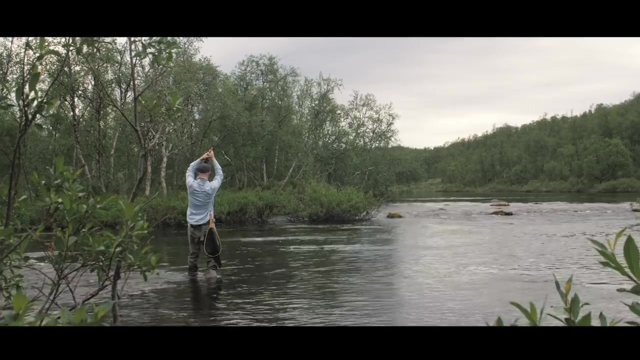 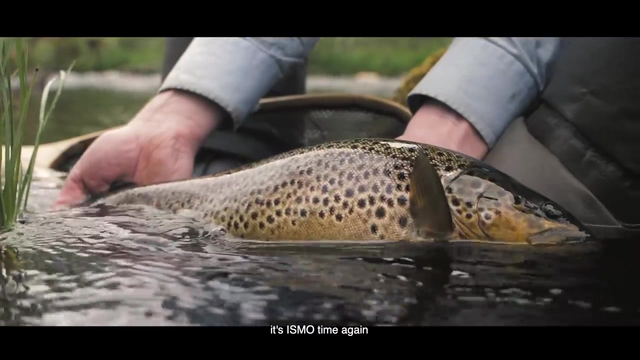 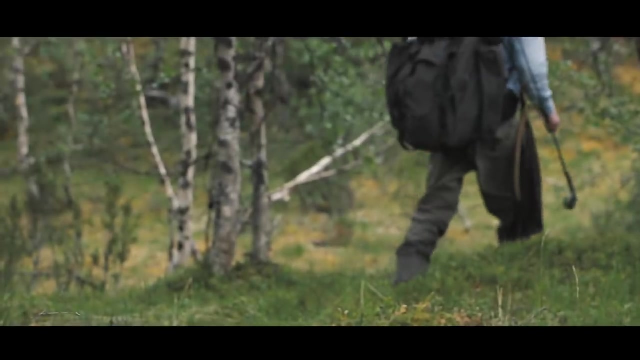 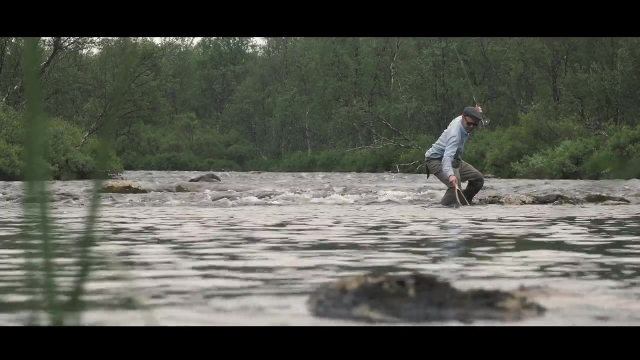 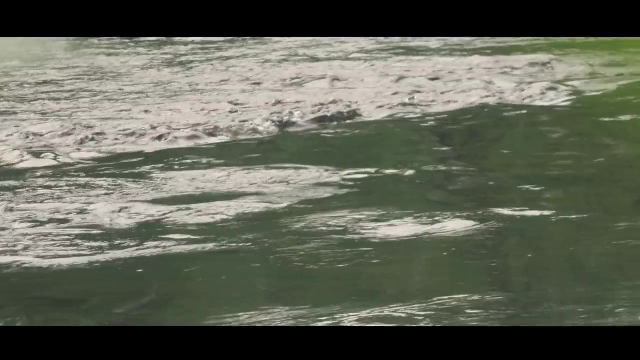 Yes, you are. That's what I'm going to do. I've never done that before. I've never done that before. It's Isthmus time. Again, It's Isthmus time. I don't know what I'm doing. I don't know what I'm doing. 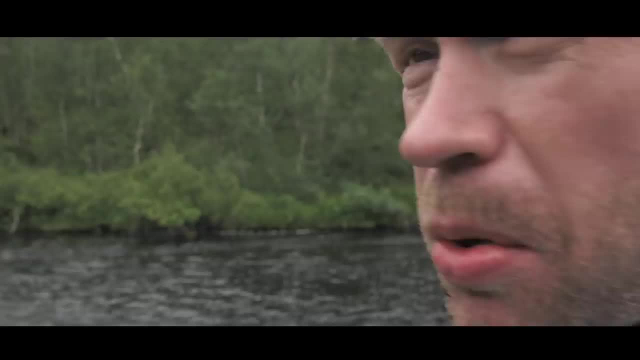 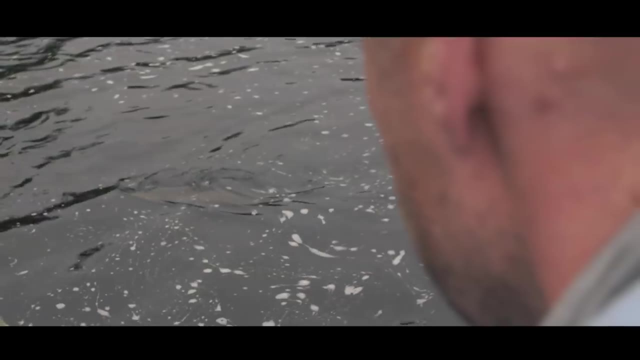 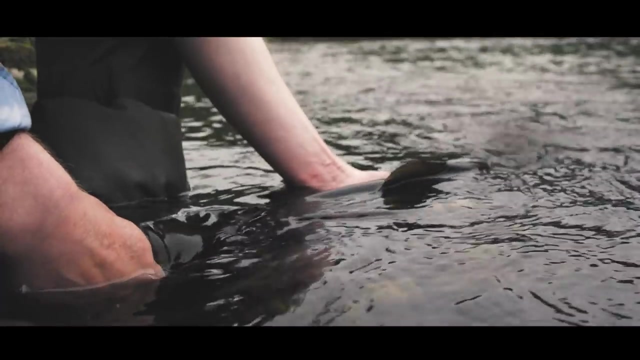 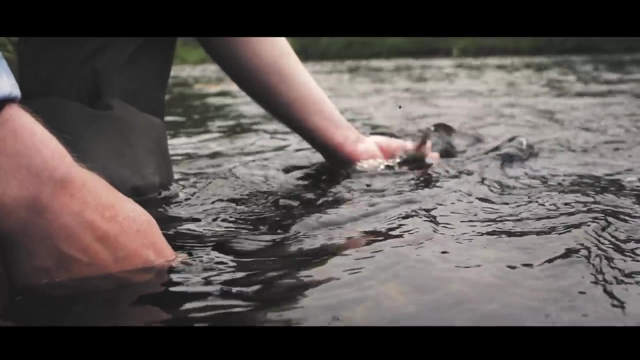 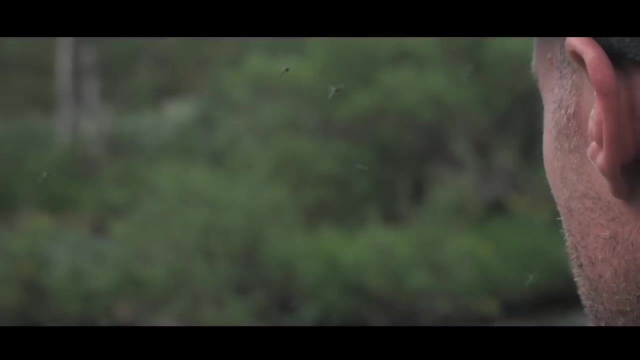 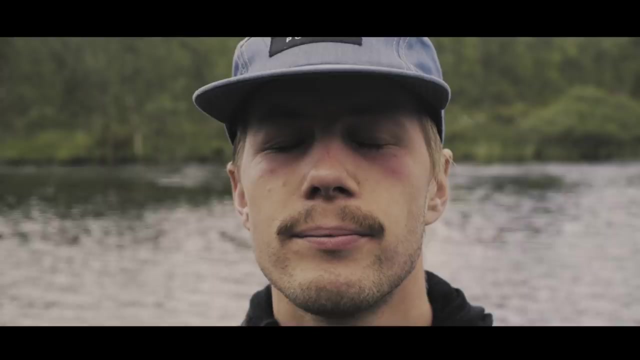 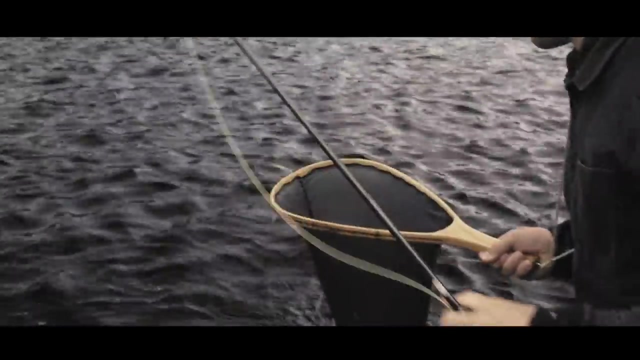 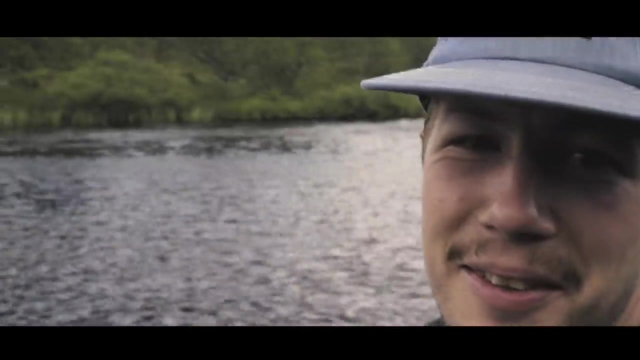 This is a big one. It's so heavy. It's a big one. I'm not sure Mindfulness. I just caught what we needed in order to survive And nothing more. I thought it was the big one that cut it. I thought you did 600 grams. You know I'm good at eating fish. 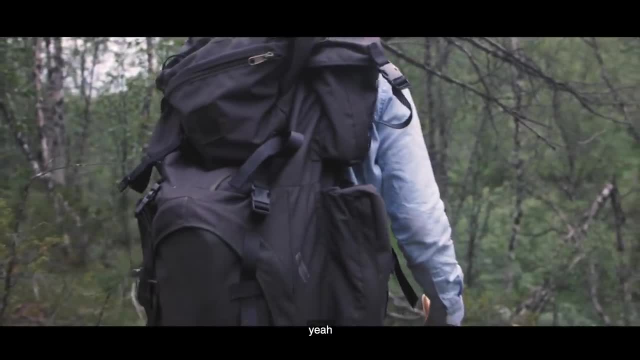 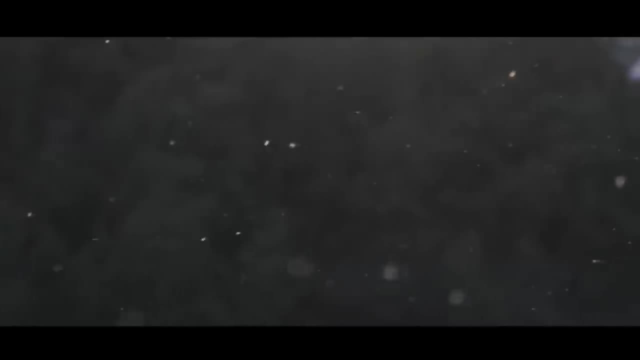 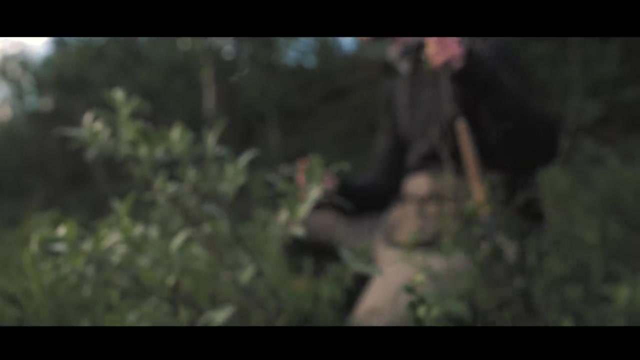 I'm very good at eating fish. You get the most beautiful fish. This is a perfect meal. Yes, Yes, At the end of the day, I was the hero, Saving us from another porridge meal Because we needed energy During the day. we had lost around one gallon of blood. 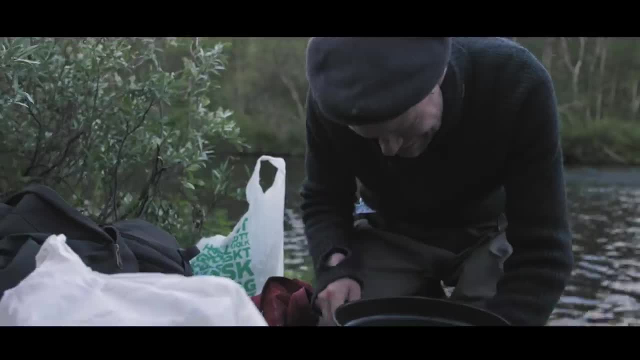 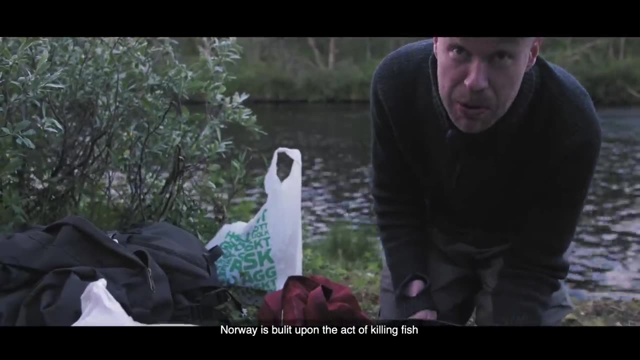 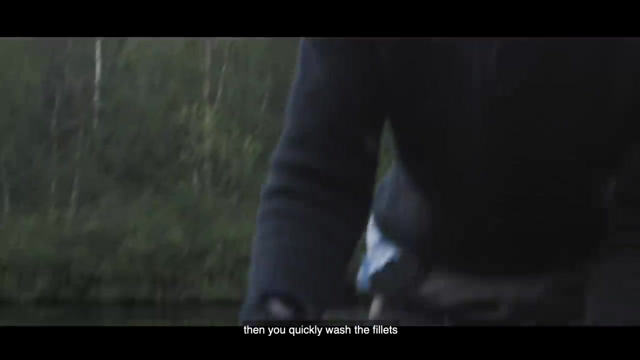 To the blood sucking devils of the arctic. It's more Norwegian to kill fish. Yes, you can say that Norway is built on killing fish. Norway is built on killing fish. And then you know, You just take it quickly and rinse it. Yes, that's the way it is. 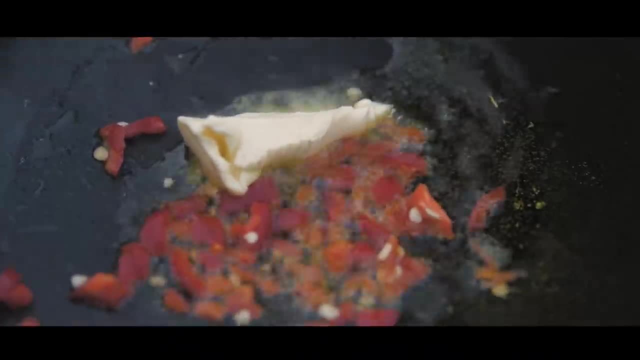 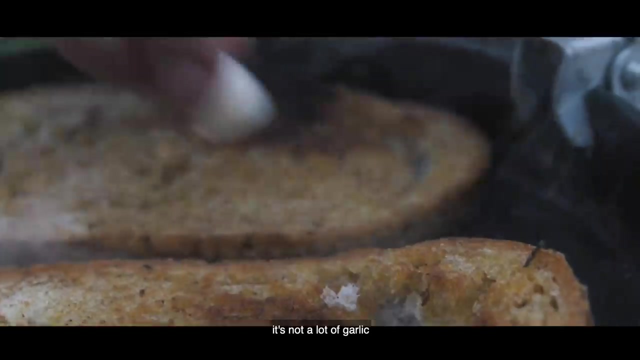 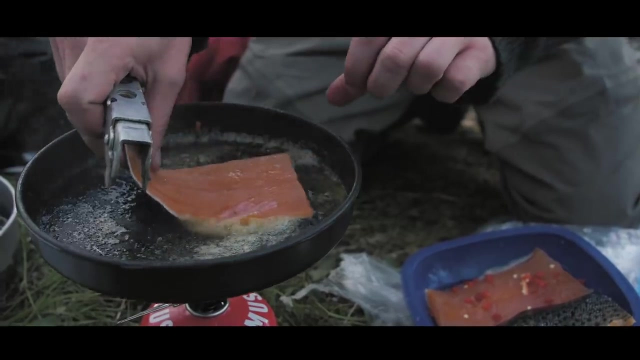 Yes, that's the way it is. Here we use a lot of flour oil. It's not going to be a lot of white oil. It's going to be a lot more than you think. This is very simple. Oops, When fishing, it is very important that it is not too much fried. 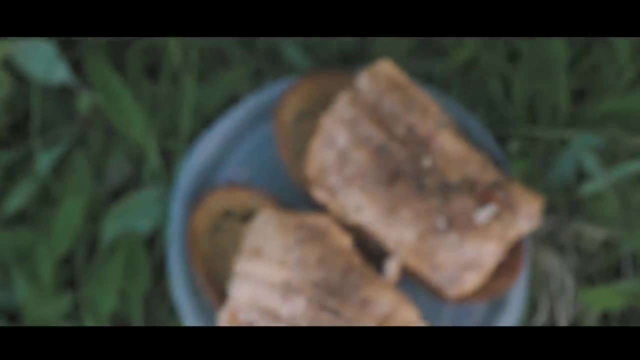 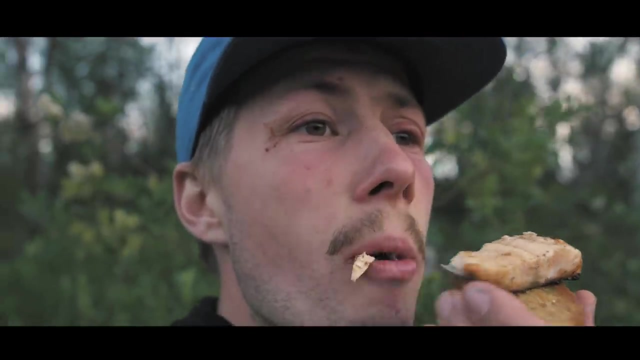 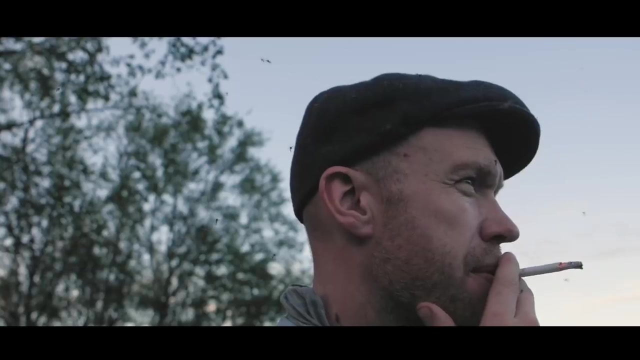 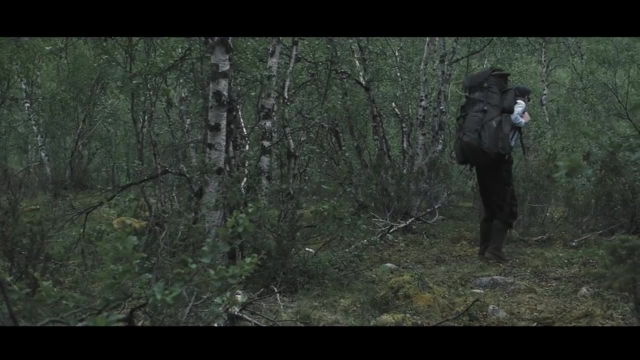 Yes, that's right. And then you just end with a little bit of the earth from the tractor. I knew it was time for us to leave, Not due to the mosquitoes And the river was still full of fish, But the fly fish's worst nightmare was approaching.